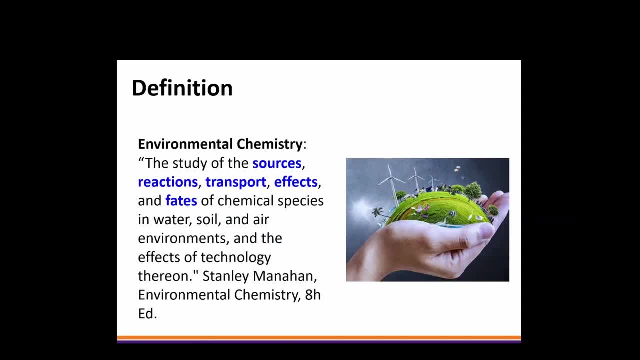 effects and fate of chemical species in water, soil and air environment and the effect of technology thereon. So it's basically, when a chemical species are emitted into the environment, we need to study where it came from, what reaction it undergoes, how is it. 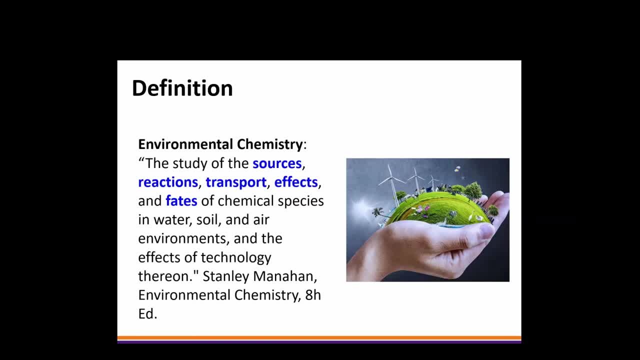 transport, in the air or in the water or in the soil- its effect to the human or to the organism, living things, and also the fates. What happens to the chemicals when it is emitted to the environment? So, for instance, they tend to a few processes that it can undergo, for example bioaccumulation. 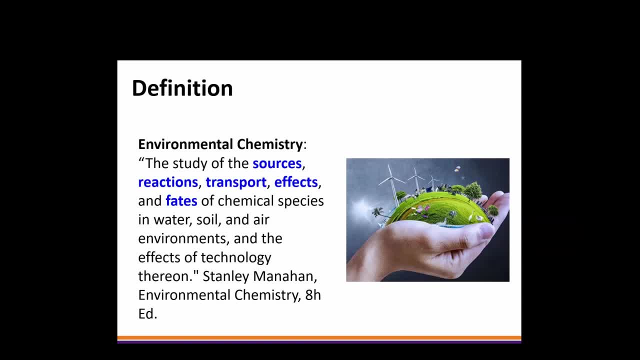 biotransportation and so on. So we will discuss what happens in the environment and then the effect of technology With the advancements of science and technology. so now we have to consider this technology. What can we? what he has done so far, the technology, what? 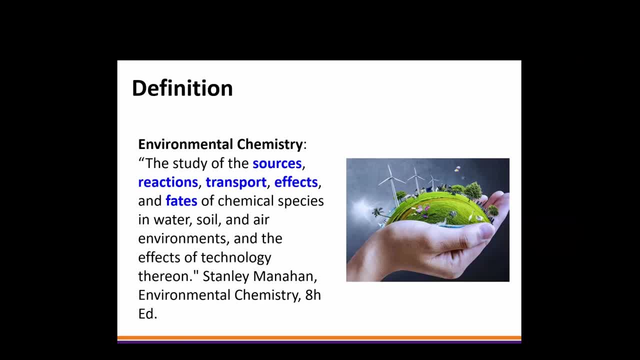 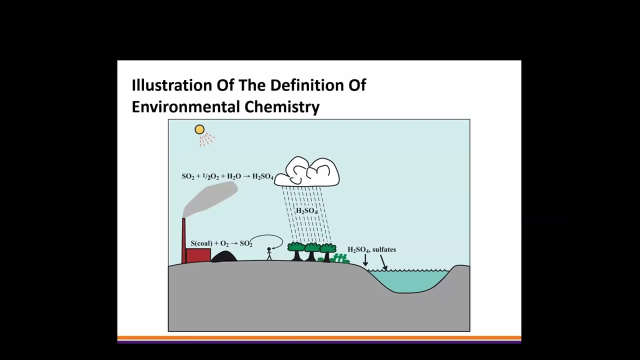 he has done so far, the technology. So now we have to consider this technology. What can we? what he has done so far, the technology, what he has done so far, the technology. what can we, what he has done so far, the technology, what he has done so? 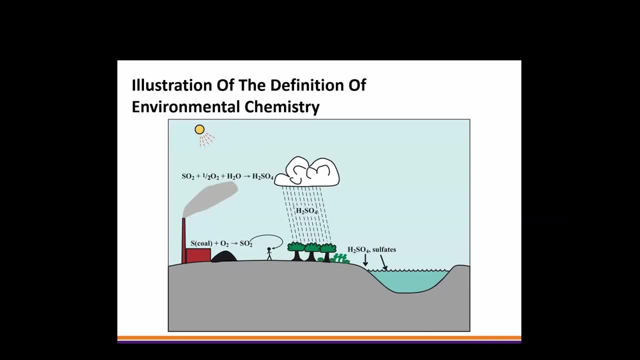 basic chemical reaction that can occur in the environment. so in this case we have a sulfur. sulfur that is emitted from a smokestack: okay. from factories: okay. now it's emitted into the atmosphere. sulfur comes from coal burning: okay, and then now it's emitted into the air. 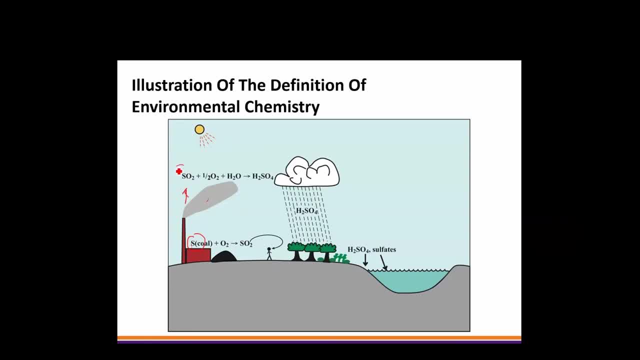 to the atmosphere and then it oxidized to sulfur dioxide. okay, so sulfur dioxide is considered as air pollutant. it can affect the human uh respiration and also it is toxic to plants. okay, or it's phytotoxic, it's toxic to plants. so, uh, in the atmosphere the sulfur dioxide is then. 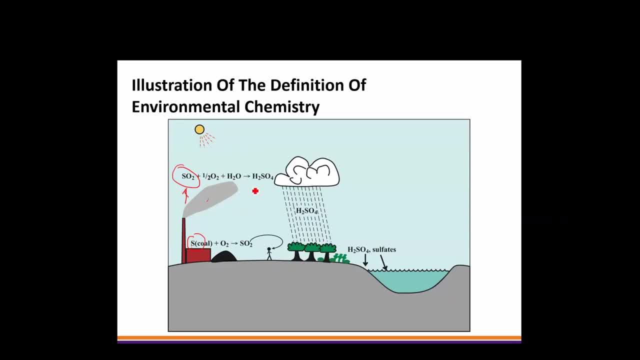 it can react with oxygen and water to produce is sulfuric acid. okay, sulfuric acid is considered as uh- acid rain. okay, when it reacts and then it forms in the cloud. when it deposited into the uh, into the land, it uh it's, it's considered as. 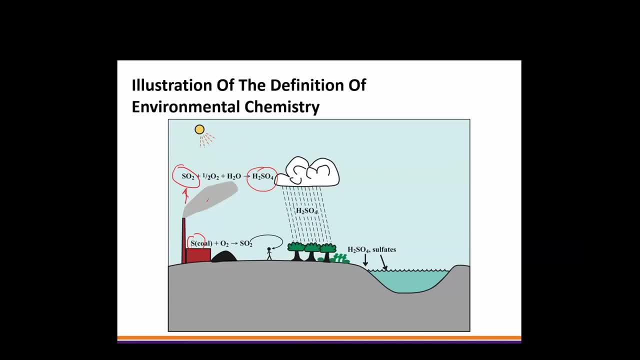 acid rain, because it's very acid, and then when it's deposited, uh, into trees, plants and everything, uh, these are considered a sink, okay. sink, okay, it can be either a plant or land or human, or it can also be sink into the water, okay. so, uh, now, once it enter, okay. 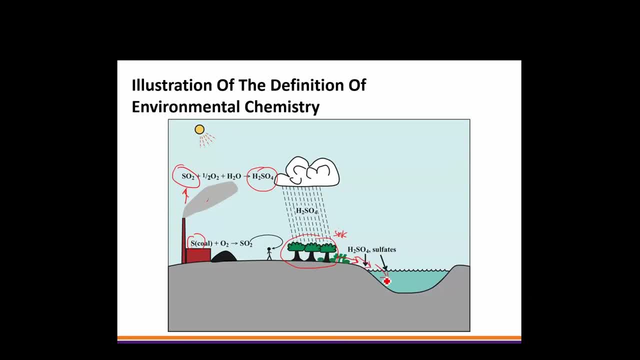 the sulfuric acid enters the water system- uh, it can be lakes or sea and so on. so this sulfuric acid, uh, will be turned into sulfate. okay, so this is the reaction that shows uh from uh, the transformation of uh chemicals from a source- sulfur- to sulfur dioxide, to sulfuric. 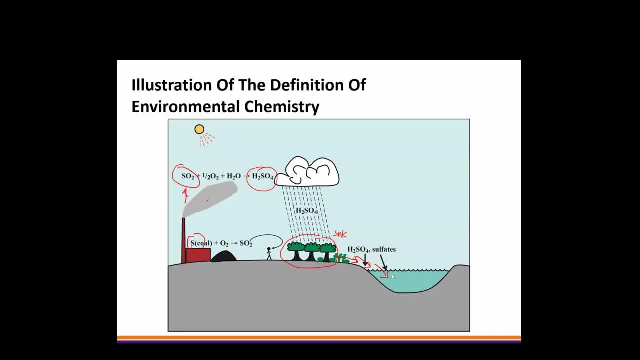 uh sulfuric acid and then finally sulfate. so if even sulfate can undergo, it can recycle back uh to the uh, it can be uh deposited or it can uh seep through the uh, the water system, to underground water, for example. if you have underground water here and it can seep through. 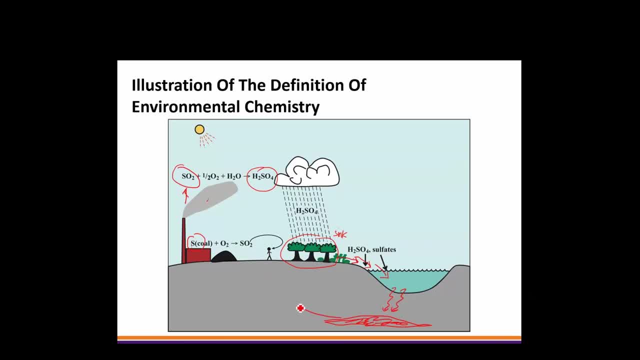 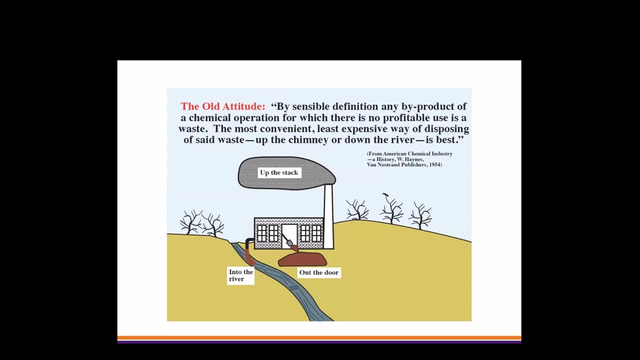 through the underground water and then underground water is consumed back to the human it is. it's a process where, uh, it is affecting the what atmosphere? the atmosphere, the hydrosphere and also the lithosphere. okay, uh, previously in the past, uh, there were many environmental problems that are caused by the. 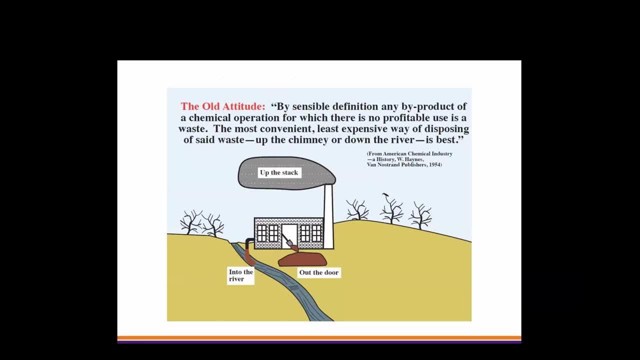 practices that, uh, now we see in our communities it as unacceptable. okay, so, for example, this is the old attitude. this is according to the american chemical industry by a historian in 1954. it says that, by sensible definition, any by-product of a chemical operation for which there is no profitable use is a waste. okay, so the most convenient. 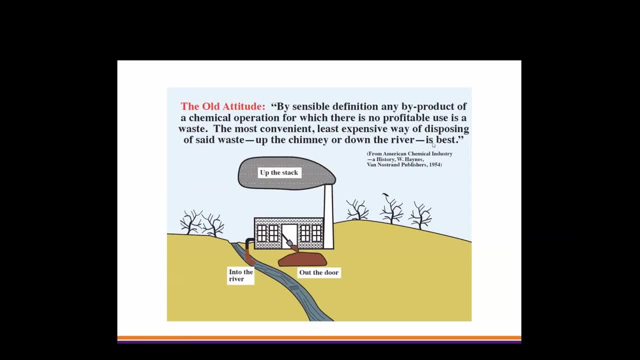 least expensive way of disposing of the said waste is up the chimney or down the river, and it's the best method to dispose this waste. okay, so can you imagine in the 1954, 1954, this is what they have been. uh, thinking, or the way of thinking, is that whatever is a waste, we can eliminate them by. 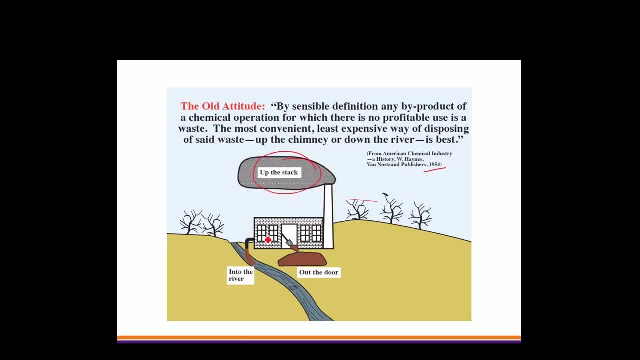 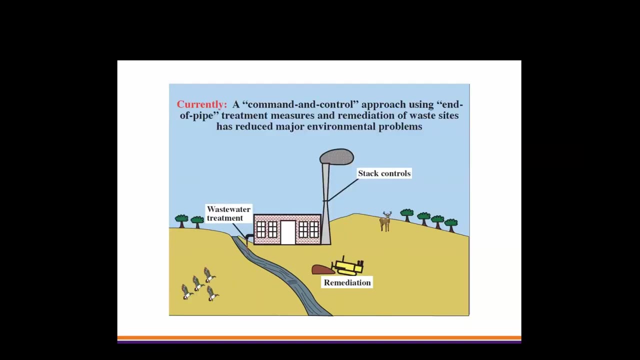 disposing it through the chimney and also down to the river. okay, they said that this is the way, but now we know it is not the best way. it's actually the worst way. okay why? because now, in starting 1970s, they have seen that the effect of these ways being emitted into the environment, and that is when 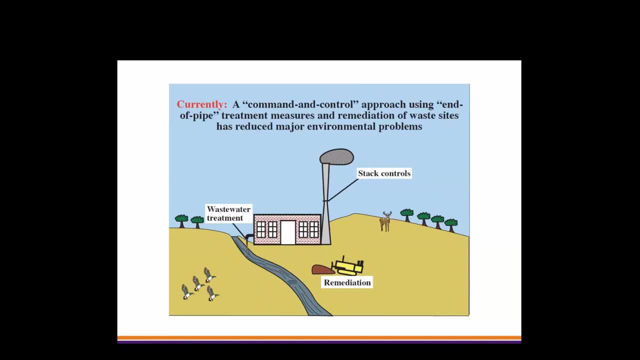 laws and regulation been implemented to control air pollution and also water pollution, and we can uh they have been methods to clean hazardous waste sites. so that's mean that uh, the solid waste and so on, they have been measured. uh, the aim now is to uh even eliminate the waste at the end pipe. okay, now. 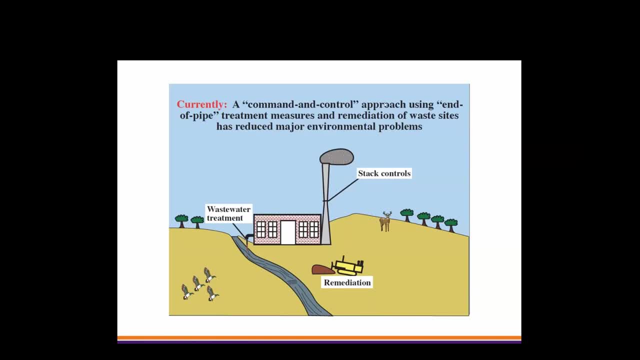 there is a uh, a command and control approach using end pipe and of pipe treatment measures and remediation of waste site has reduced major environmental problem. that's mean that now uh, before we can emit the uh, the waste, we have to control the waste so that now the factory have 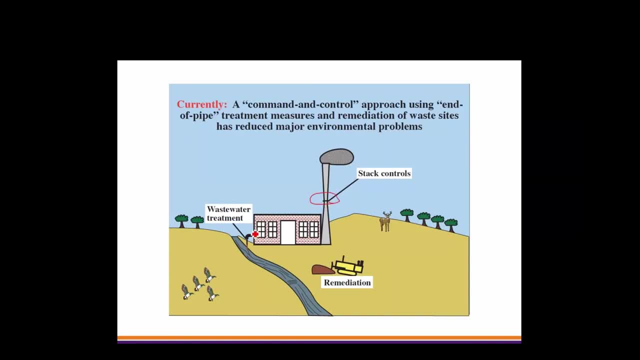 to implement stack control, they have to do a wastewater treatment before they dispose, and then they have to do remediation for the solid waste, and so on. uh, but one thing disadvantage about this technique is that it's costly and it requires constant surveillance to make sure that. 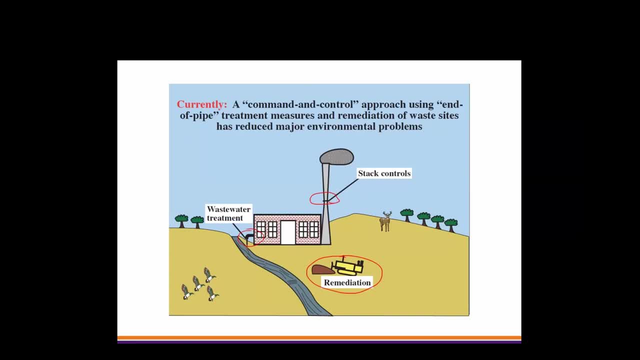 the standards are meet and that uh this have been uh so that we can reduce the amount of waste emitted into the environment. so this technique has been reducing uh pollution and has prevent the increase of uh, a pollutant release, but is costly and require constant uh surveillance. 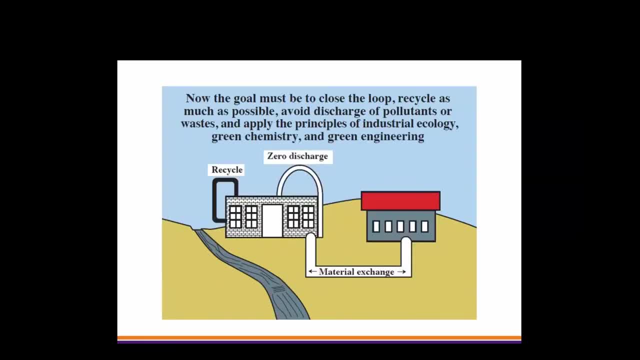 okay, so what now? the goal is that we have to close, close the loop. okay, so that, uh, we must recycle, recycle as much as possible, avoid discharge of pollutants. we must avoid and then apply the principle of industrial ecology, green chemistry and green engineering. so this is what we'll, we are working towards: we have to recycle, we have to create zero discharge, and then 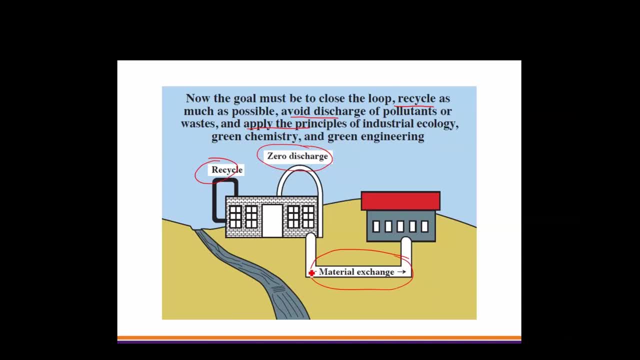 uh material exchange, material exchange meaning that maybe we can uh from waste to wealth. i don't know whether you have heard this concept or not. from where uh waste to wealth? okay, so that whatever waste that is uh produced from a factory or industry, we must be able to change that into something that is profitable, that can generate income. 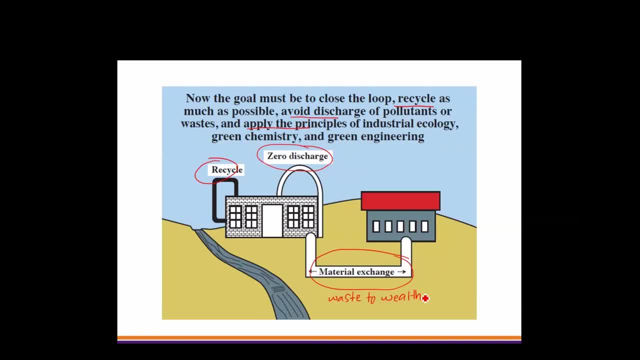 for example, burning of coal, okay, or cold, okay. so that, uh, now how can we generate, or how can we reduce the use of coal burning coal in burning to generate, uh, energy, or to generate heat, okay. or from agricultural waste, for example, uh, from coconut, okay, how can we.